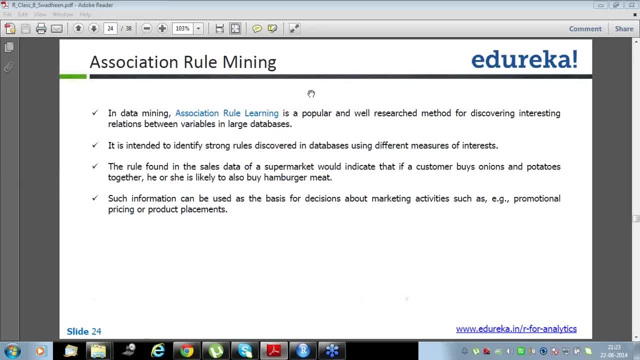 that if a customer buys onion and potatoes, together or not, He or she is likely to also buy hamburger meat. That's what the association help us And, based on this analysis, things can be put together or nearby. Such information can be used as the basis of decision about. 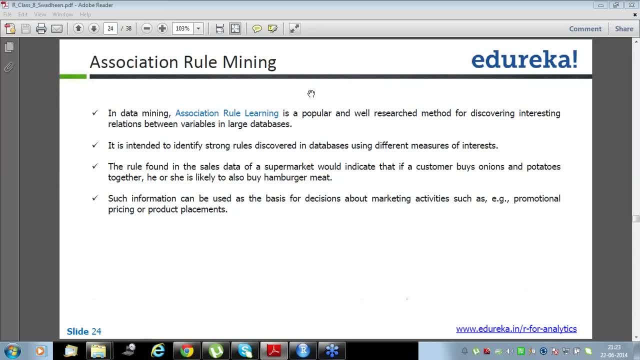 making activities such as, for example, promotional pricing or product placement. And there is one more aspect of association rule. Association rule tells you that which two or more products are more closely related. But you know we are using association rule in finding the frauds where we know I am using 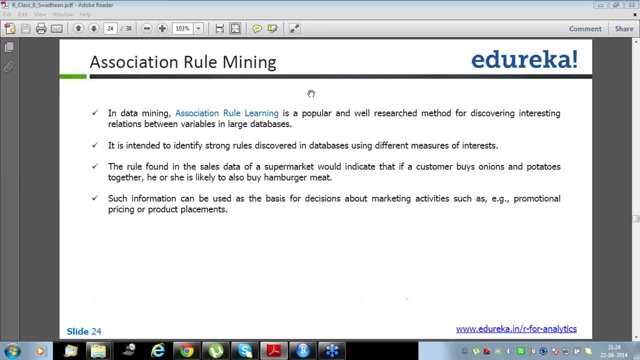 this technique in an opposite way. I am trying to figure out within the disease that which are the disease could lead to, or which are the disease codes have. the more association I mean which are two or three disease codes could lead to. The other disease code, higher disease code, right, But if I got to know that some disease 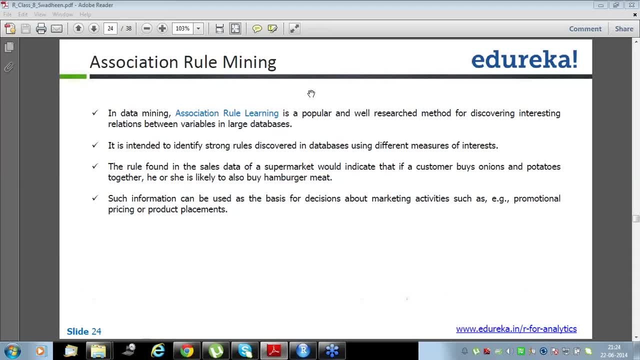 codes have less association or very less association. I mean they must be apart And some of the doctors are building these two codes together. So where the alarms situation comes, And we thought that definitely there must be some, And if the frequency is more definitely there, 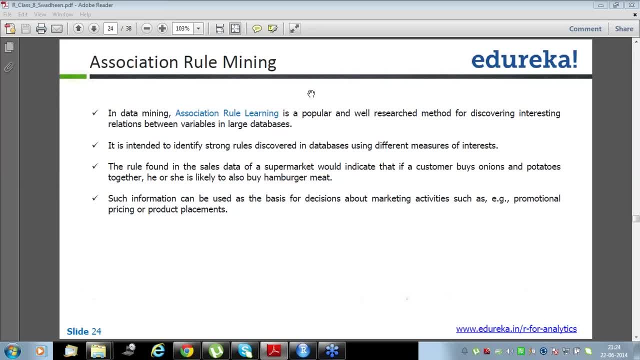 must be some fraudulent activities happening. So association analysis helps in both the ways It gives you the association or the liking grouping between two values And also if two things are not really correlated. they also explain you many things, Because I told you decision, what decision you need to take. 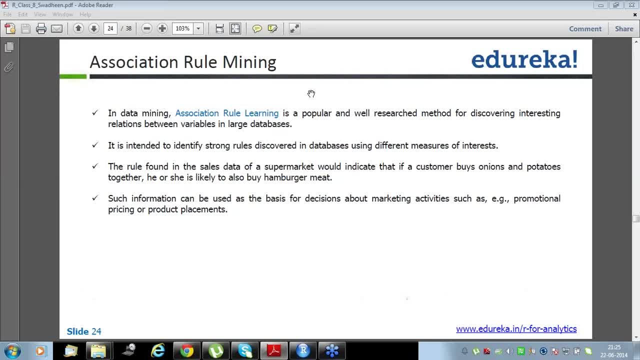 depends on your understanding, right? Yeah, Abhinav, it's very interesting. Yeah, Like. working on these concepts has really, you know, revealed many of the things. The rule found in the sale data of a supermarket would indicate that if customer buys onion, 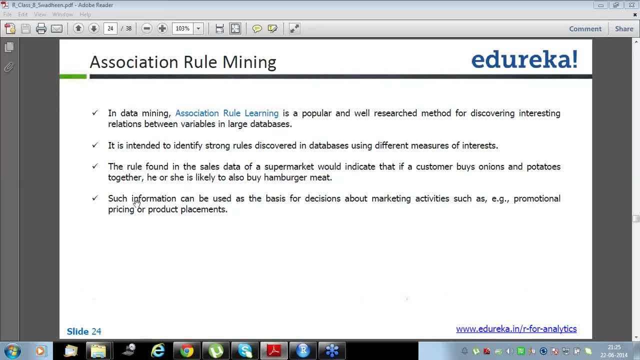 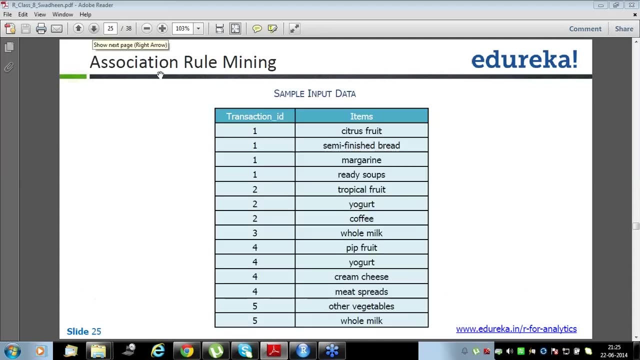 – oh, I covered that Such information can be used as the basis for decision about marketing activities, such as promotion, pricing or product placements. okay, Okay, So let's say we have a transaction ID, Transaction ID. I see one means like. it is like it. 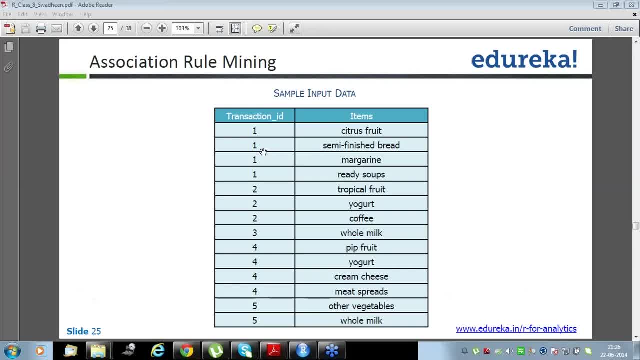 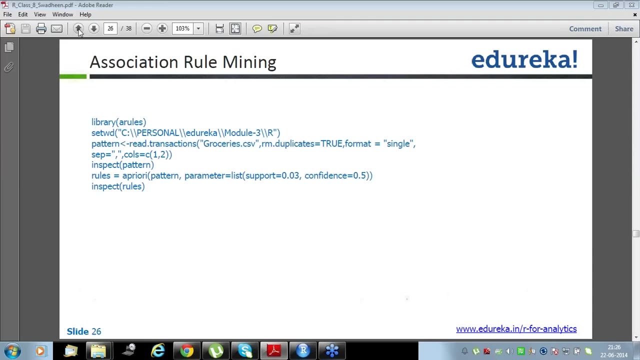 is a bill of person. A buys these four items – citrus fruit, semi-finished bread, margarine, ready soups And two. a transaction ID 2 has three items like three. these three items bought together by other person. Similarly, in the third transaction only whole milk is. 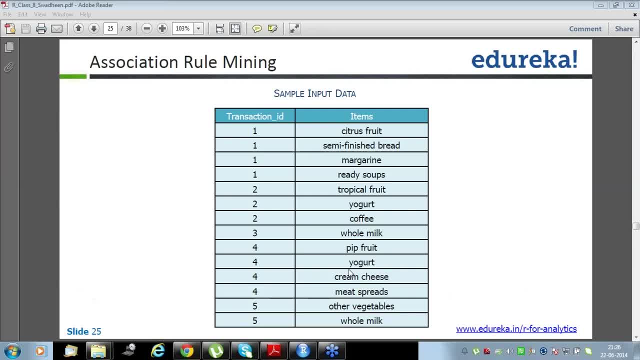 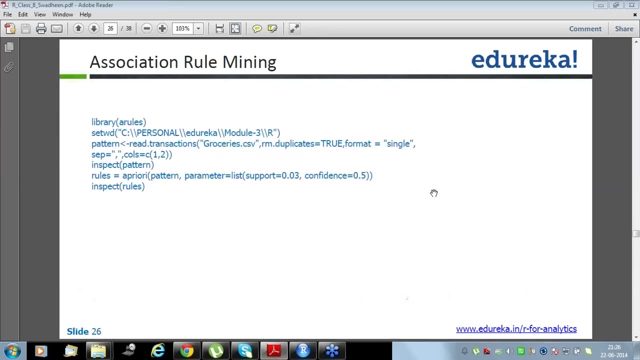 bought, Like the one person bought only whole milk In the fourth transaction. let's say, this is the transaction ID of a day or a month maybe. So that's something. your input data is Okay. Yeah, Okay, that is something. But before working on that, look. look here, Like rules equals. 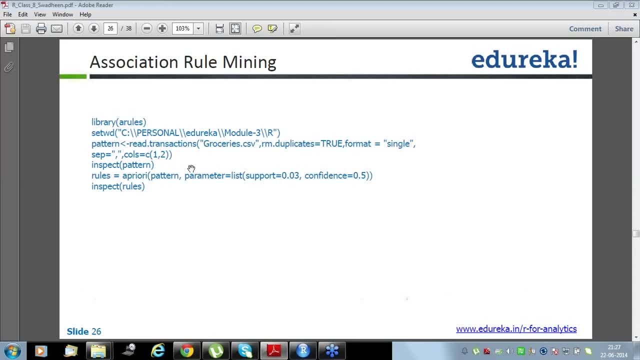 to a priori pattern parameter list. support and confidence. What is the support and confidence and lift? So be very attentive here. It's very important concept. Until, unless you don't know about the support, confidence and lift, you cannot take any decision. 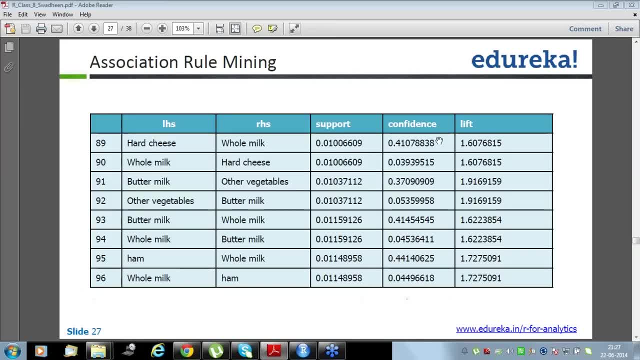 Even you cannot read the association rules, So like the association analysis would be in something like in this way: Hard cheese and whole milk support 0.01,. like 10%, It has a confidence of 0.4107, so approximately 41% Lift is 1.60%. Important is – What? 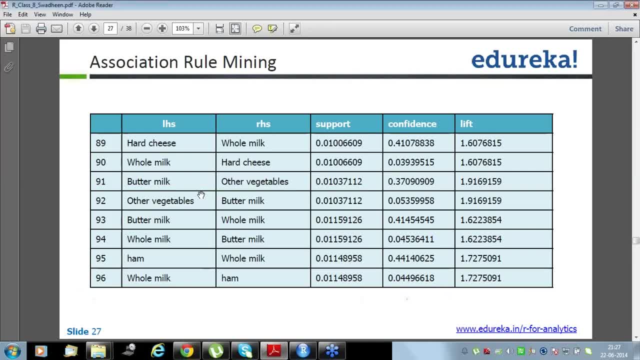 is the support confidence lift reveals. What does that mean? Do we need to understand? what does that? orpieces into a connection function, Literally, you see, when you put like they're not very much important. so it's very much important to understand that. 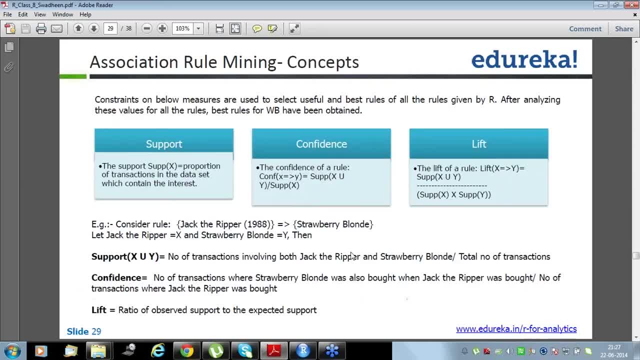 what is support, confidence and lift? Look at here. can you see that this one, okay. Support is equals to proportion of transition in the data set which contains the interest. Actually, it is what it is: the probability of item A out of the total data set. You got my point. Like, let's say, 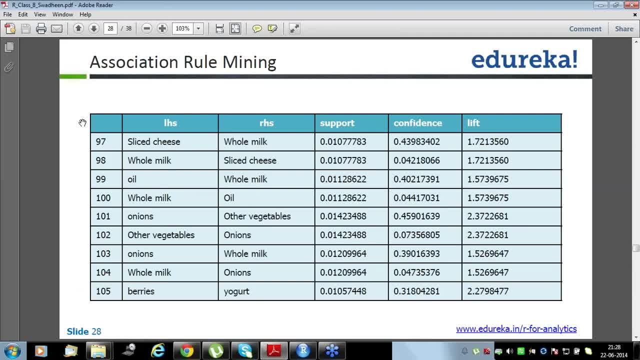 for example, we're talking about the rule number 97. in rule number 97 is saying that slight cheese and whole milk. So whenever slight cheese is bought, whole milk also bought. With support 0.01 percent, confidence is 43 percent and lift is 1.72 percent. 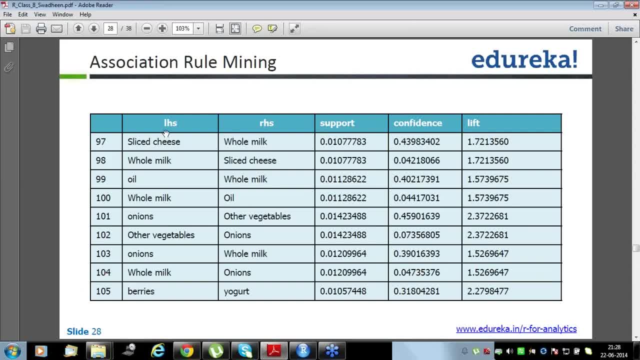 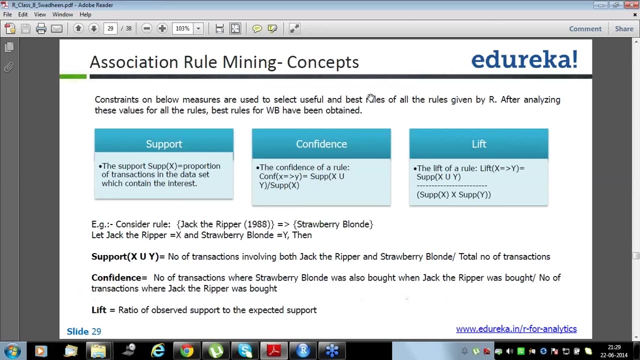 What does that 0.01 support mean? Support is always for LHS side. That means out of the total data values, slight cheese is bought, only 1 percent of time. You got my point. Look at that. Support is what Proportion of transition in the data set which contains the interest. 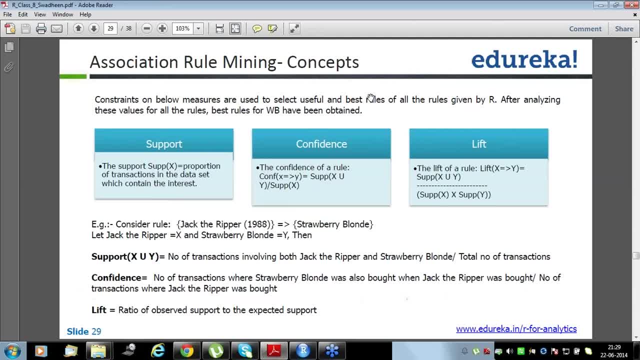 So let's say there were 10,000 items bought in a 10,000 different items bought in a day or in a month. So let's say this data is for a month. So out of those 10,000 times 10,000 items bought in different transaction. 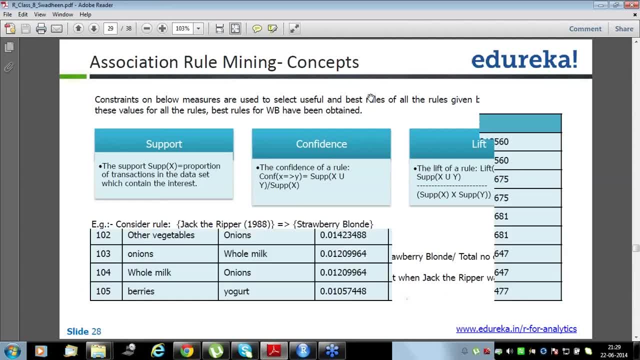 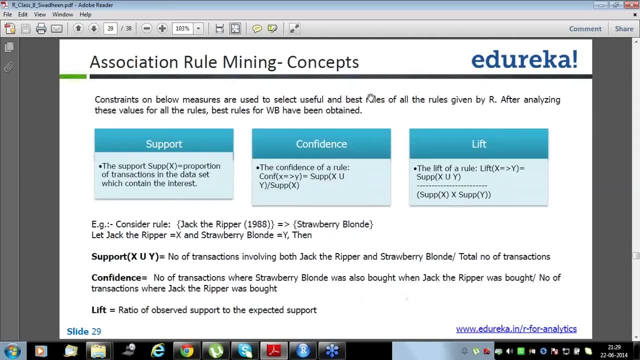 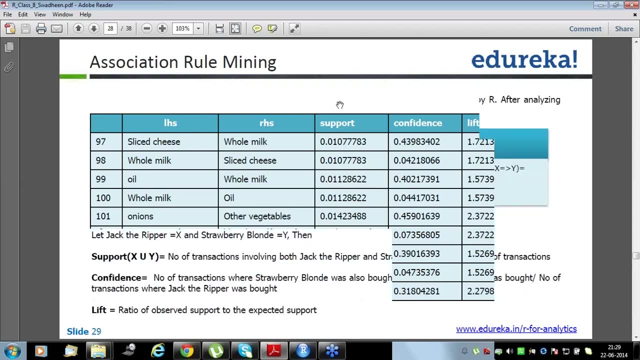 in a month only 1 percent. So 1 percent is around 100.. 100 items were slight cheese. Are you clear with that? Support is what? Support is always for LHS. Look at the LHS side Right. Second is confidence. Confidence is always. look for the RHS side. 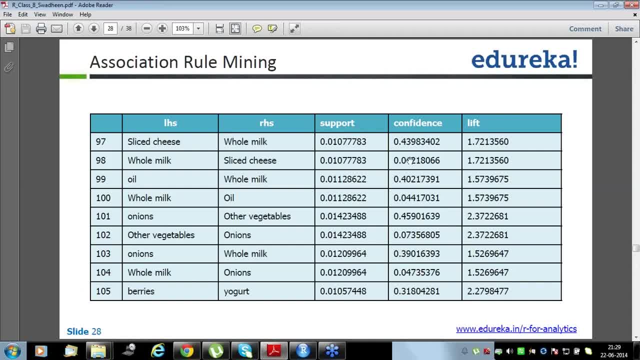 So this RHS if you look at the confidence: 0.43 percent. So now how you would read it. Like you look at slide cheese and a the whole milk. We know that whenever the the slide cheese is bought, Whole milk also bought. 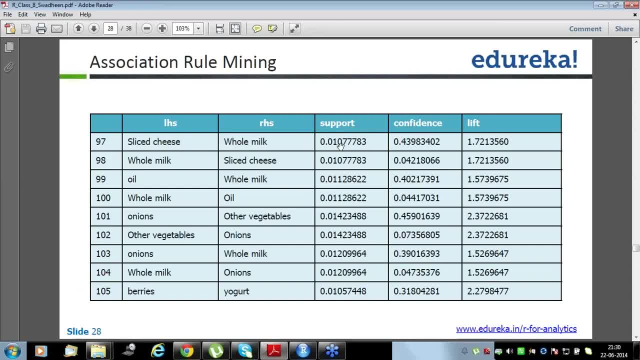 But slide cheese is bought only 1 percent of time. That means out of 10,000 items. So you have it all. 0.14 percent is 9.62 percent. Only 1 percent is bought into the SID sense names chart. 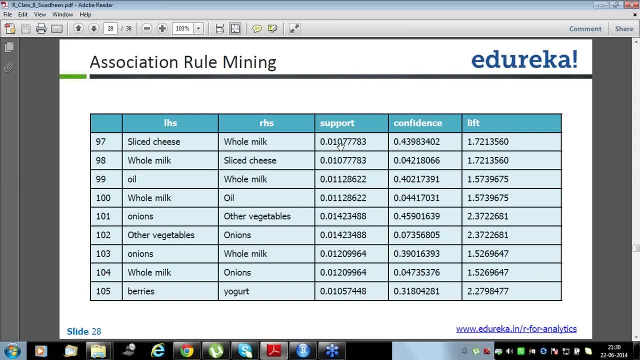 That means out of 10,000 different items, slide cheese is bought only 100 times And out of those 100 times, 43% of time whole milk is also bought, Like 43 times slide cheese and whole milk bought. 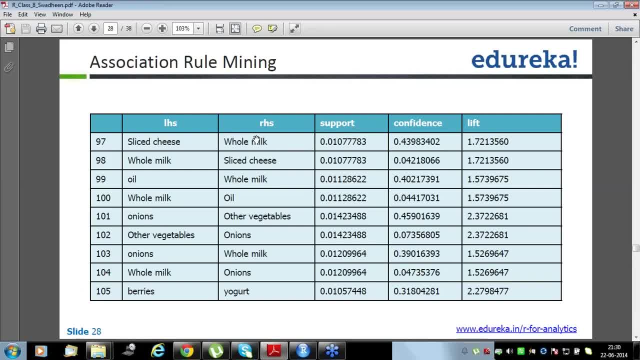 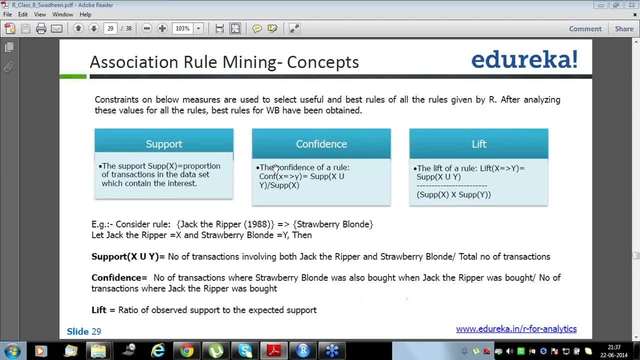 together. Confidence is for whole milk when it bought together with slide cheese. Now look at this confidence. How this confidence is calculated. The confidence of a rule is equal to supply of X union Y divided by supply of X. That means probability of X and Y bought. 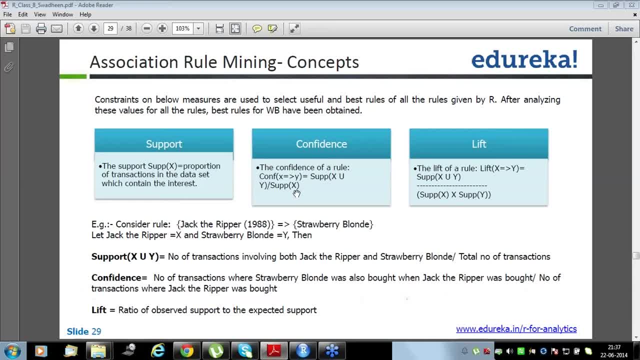 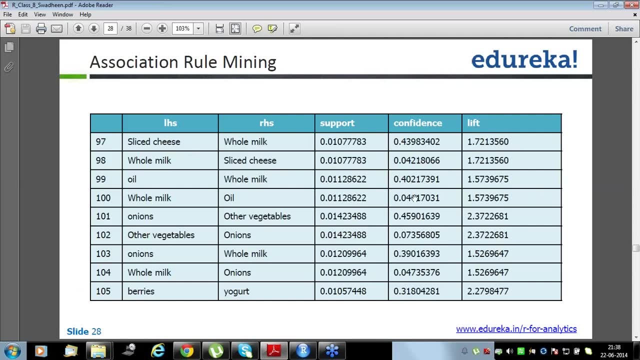 together divided by probability of X. The confidence is that actually It is the probability. It calculated in this way. Okay, Right. So look at that. If you look at row number 101, how this confidence is calculated: Probability of buying onion and other vegetable together divided by the probability of buying. 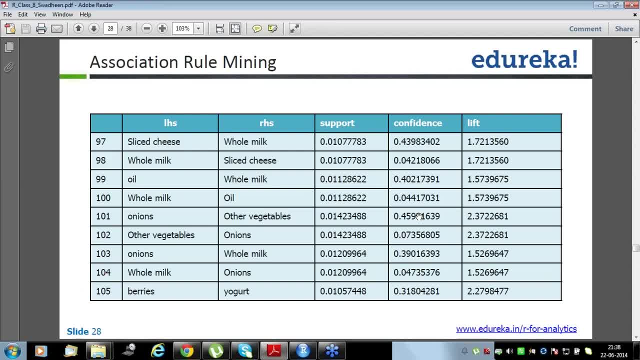 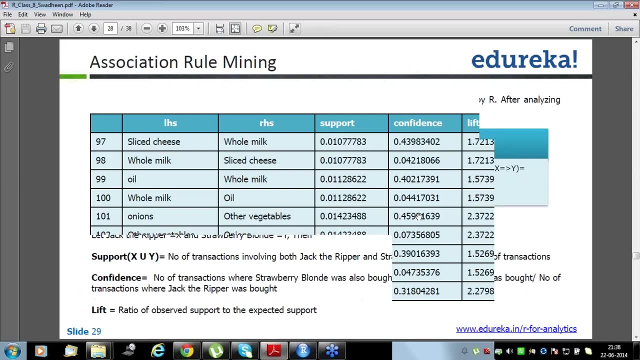 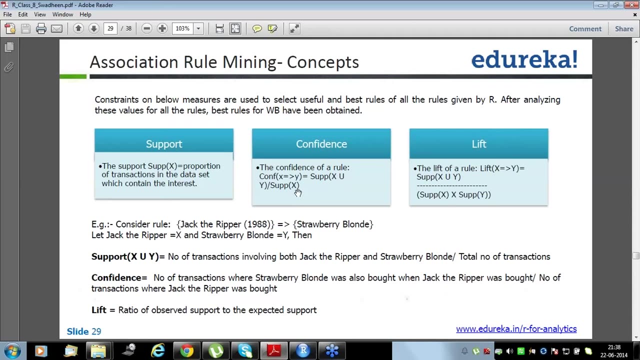 onion, Okay, And what is 102? Other vegetable and onion together divided by the probability of other vegetables. So in this case, like, support of the denominator case is equal Right. The denominator, the numerator is the same. Okay, Numerator is the same, but the 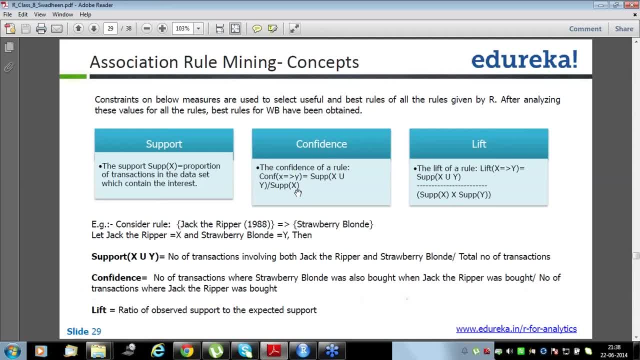 denominator is changed. Okay, Spend a little time over that, It will come in. You will clear it when we move on with more examples of that kind, Because it is the support and confidence is always is a probability value. see, a support and confidence. it would never be more than 1 and less than 0. It will be. 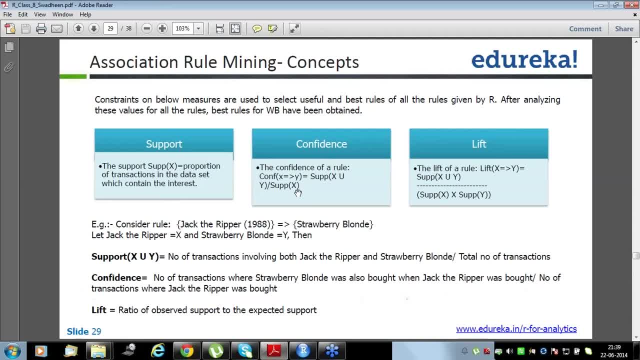 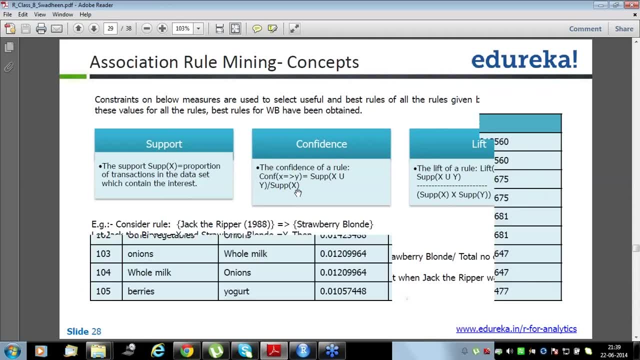 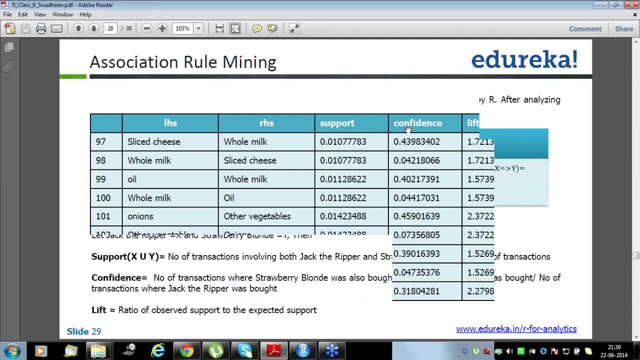 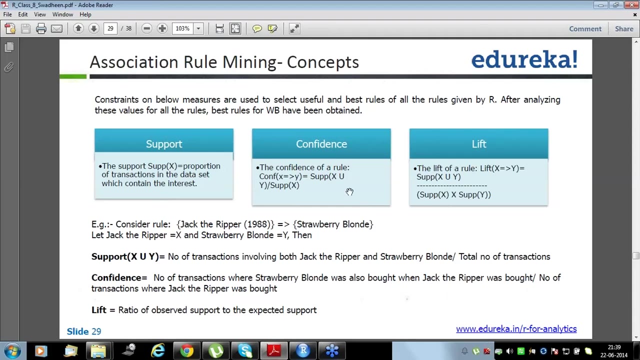 value between 0 to 1 because it's a probability value, Right? So whenever you see a support, support is always and confidence is always between value 0 to 1 because they are probability, They are calculated through probability. Okay, Now look at that Constraint below measure. 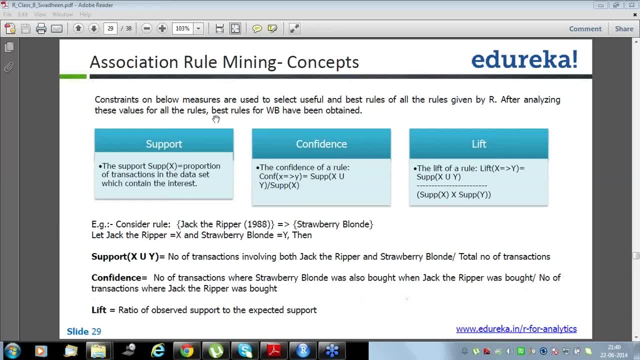 are used to select useful and best rules of all the rules given by R. After analyzing these values, for all the rules, best rules value have been obtained. Lift is what? Lift of X to Y is what Support of X and Y, X and Y brought together, divided by support of X into support. 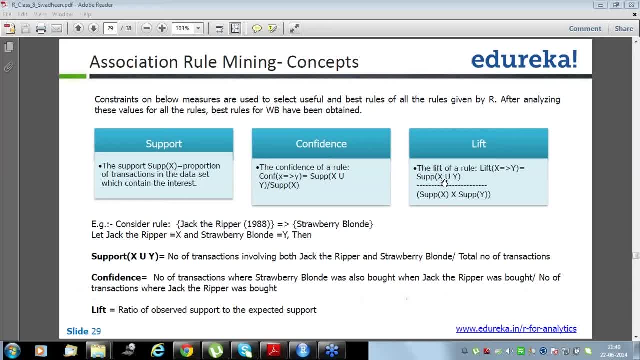 of Y. So that is the lift. Okay, So what I can say, lift is something: confidence divided by support of Y. I can say that in this way as well: Confidence something, what? How? the confidence calculated mathematically. Support of X and Y divided by support of X. How the 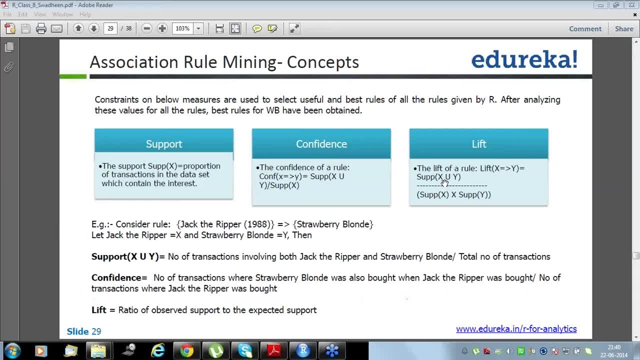 lift is calculated: Support of X and Y divided by support of X, multiplied by support of Y. Well, even I can say in this way that lift is equals to confidence of X and Y divided by support. Support of Y, Right. So just you know. spend a little time over it. Support is number of. 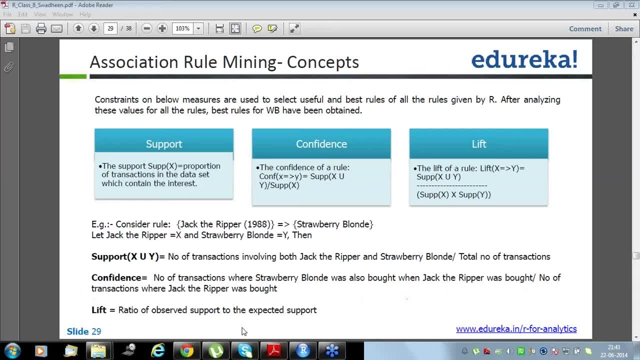 transition involving both jack and ripper and strawberry blonde. Like X is the jack the ripper and Y is the strawberry blonde. So support X and Y is what So number of transition involving both jack and ripper and strawberry blonde. So support X and Y is what So number. 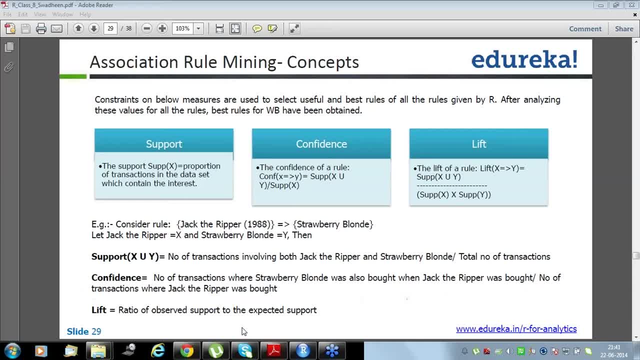 of transition involving both Jack and Ripper and strawberry blonde divided by total number of transition. That what I explain you. Confidence is number of transition involving strawberry blonde was also bought when Jack the Rippers was bought- Divided by number of transaction where Jack the Rippers was bought. So that is confidence Ratio is little tricky You. 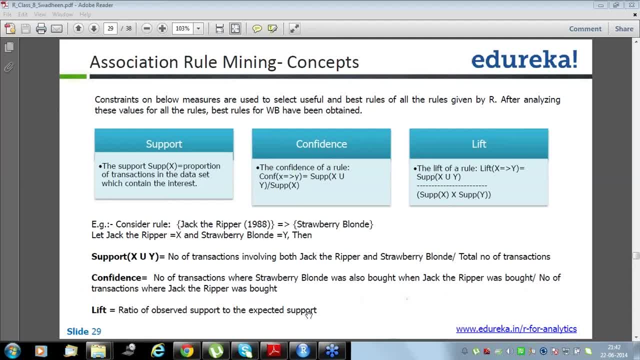 need to spend a little time over it. Lift is something: Ratio of observed support to the expected support. It would be little complicated concept. You need to spend a time over learning support and confidence. But lift, I can tell you lift is confidence of X and Y divided by support of Y. 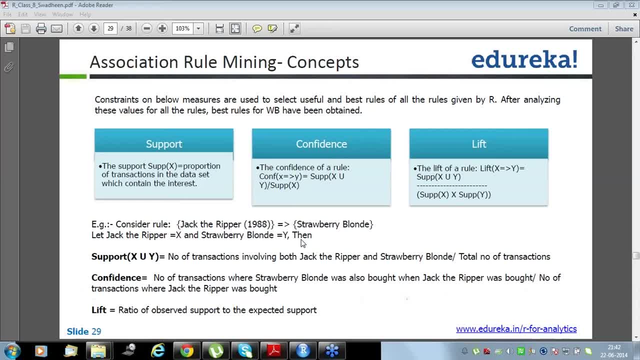 Like lift is something between X and Y. X is LHS part and Y is the RHS part. So lift of X to Y is what Confidence of X to Y, divided by support of Y, The number of transaction, the Y was there. So let's understand through this example. 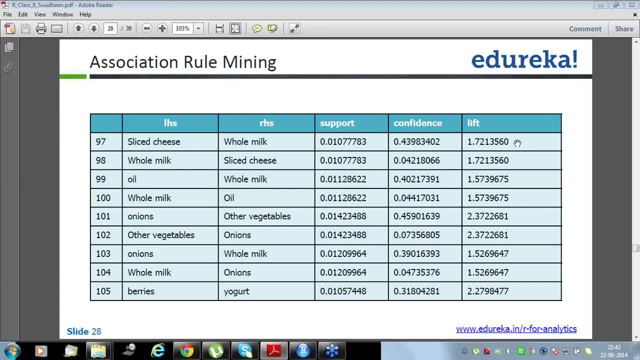 So look at row number 97.. Lift is 1.7213560.. So lift of slide cheese to whole milk is 1.72.. It means what Confidence divided by support of whole milk And how many times the whole milk is bought. 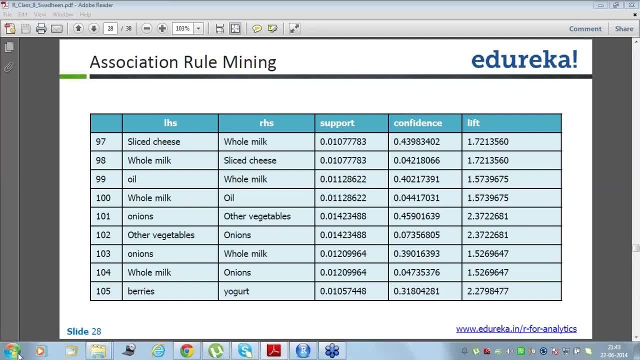 Let me do a simple calculation: 0.43983402 divided by 0.01128622.. 0.43983402 divided by 0.01128622.. Wait a minute, There is a 0.43983402 divided by 0.01128622.. 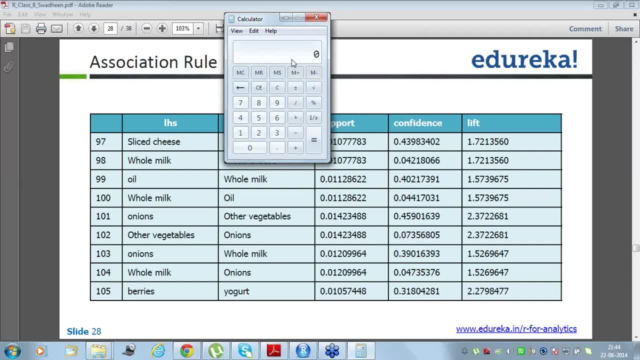 Right, Sorry. 0.43983402 divided by 0.01128622.. There is a little messed up here. 0.43983402 divided by 0.01128622.. It is good to have a high lift value. 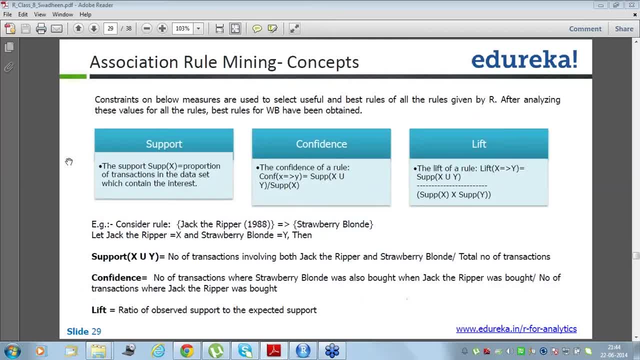 0.43983402 divided by 0.01128622.. 0.43983402 divided by 0.01128622.. So you know, look at the lift again. It is a probability concept. So that might be little messed up or little complicated to understand. 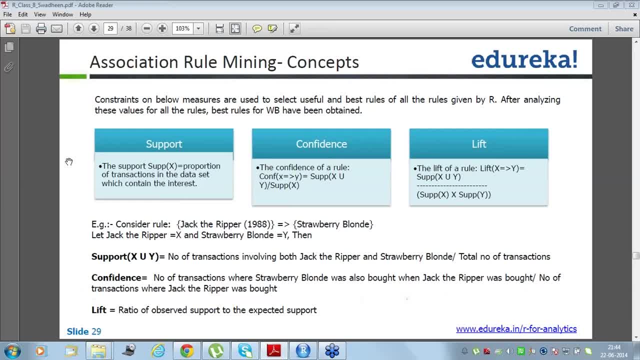 So lift of a rule, lift of x to y, is what Support of x to y divided by support of x. That is exactly the confidence multiplied by the support of y. So what I can say: Lift is equals to confidence divided by support of y. 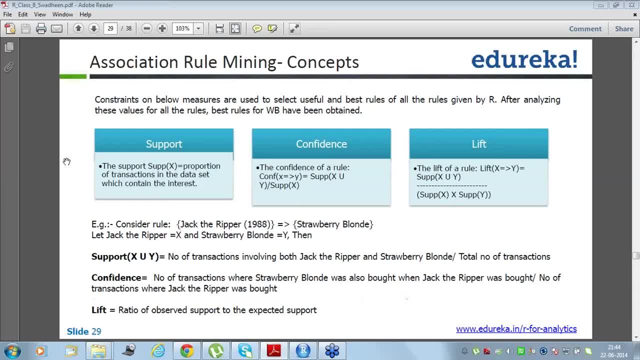 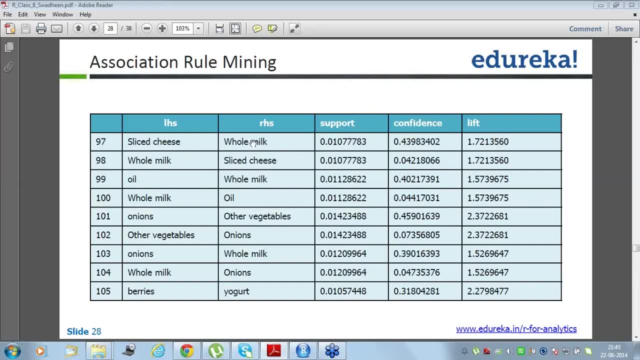 And how we read confidence. Confidence something, So confidence something. Whenever the slide cheese is bought, how many times the milk is bought? Okay, Divided by the total number of times the whole milk is bought, Okay, Okay, So high lift is good. 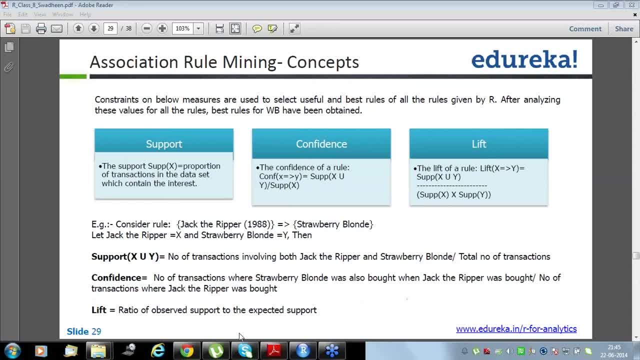 But ratio of observed support to the expected support. So it is the ratio. High ratio is good Like if you look at the definition, lift Ratio of observed support to the expected support If observed support is more than the expected support. 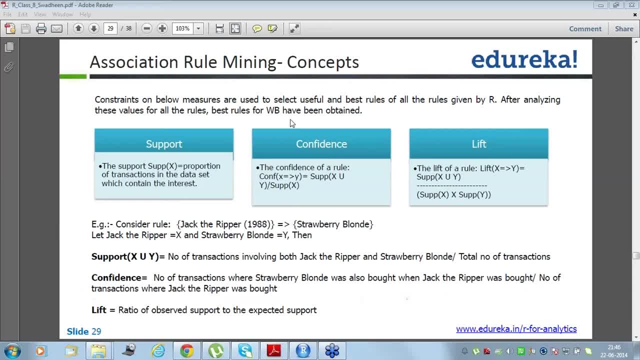 That means ratio is greater than 1.. Okay, Whenever there is observed support is more than the expected support, That means it is revealing some other phenomena. Yeah, Lakshmi, Even I think so. Let me come to the real example. 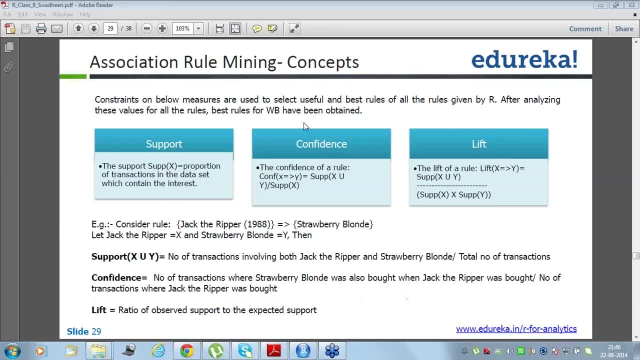 There is some problem. So let me come to that. But first let me explain you lift, Then I will probably come to the data With the R. Then we will discuss that, Because once I calculate there might seem some problem. 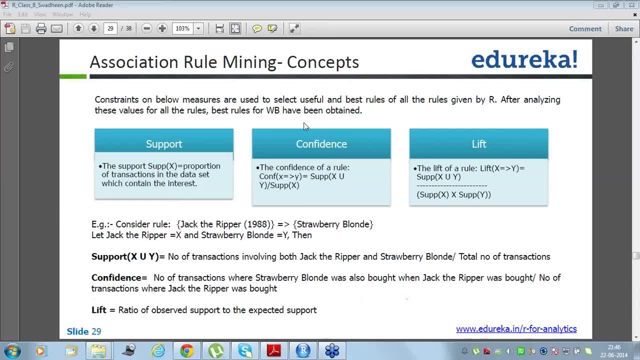 Anyways, look at the lift. Lift is what Ratio of observed support to the expected support? That means the observed support between these two phenomena is more than the expected. So sometime, what happens when lift is high Between two values? So it reveals something extra.